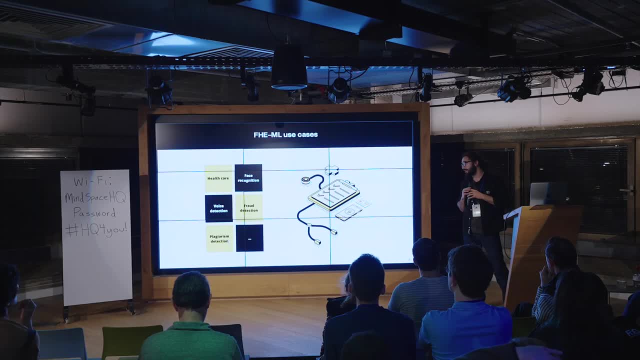 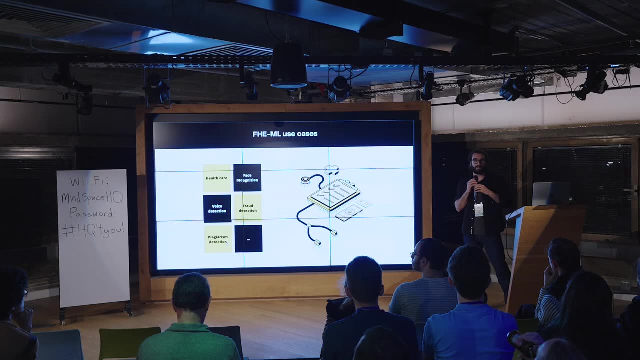 actually collect the data of the users, And that's something that you might not want. for example, if you have a- I don't know- a cancer detection model, You might not want the company that's doing that to send the data to an insurance company. 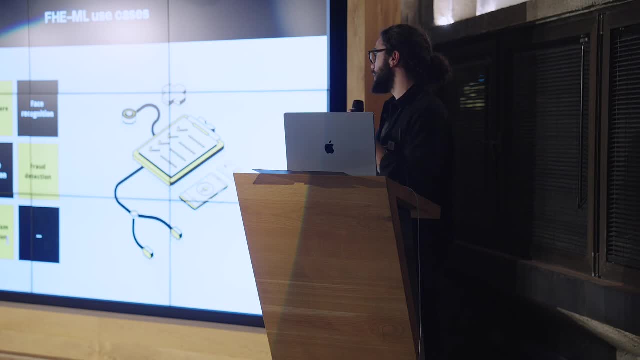 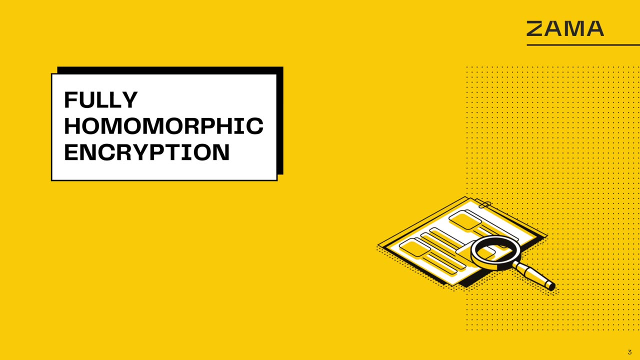 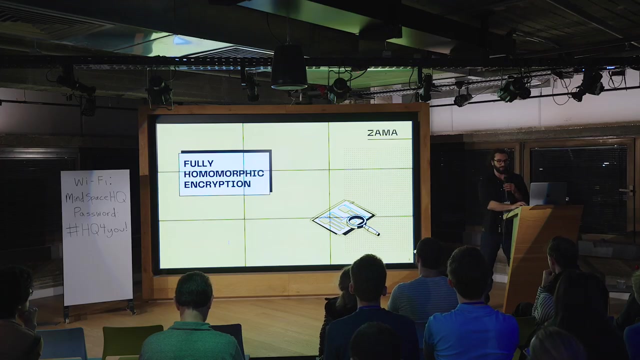 So this is why we want the model to run in FHE, so that it protects the data of the user. So yeah, first reminder of what fully homomorphic encryption is. I guess most of you are familiar with it. It's still going to do a brief introduction to it. 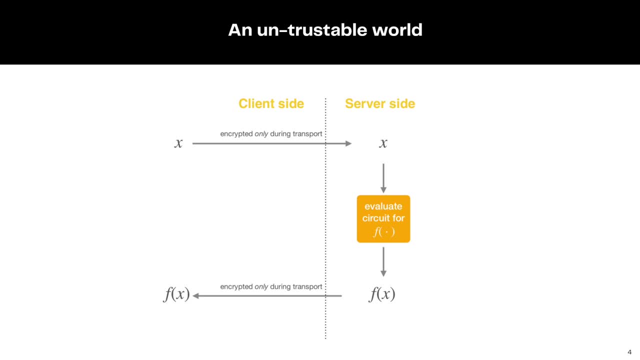 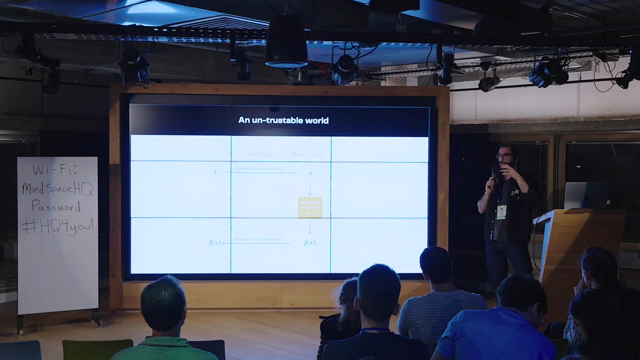 So basically, if you want, if we take the example of the World Wide Web, so we have a client and a server. The data is encrypted during transport, It's encrypted on the server side. The server does some computation or something with the data and then some result is returned to the user. 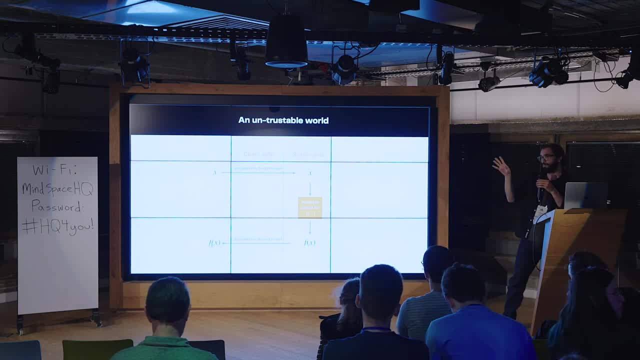 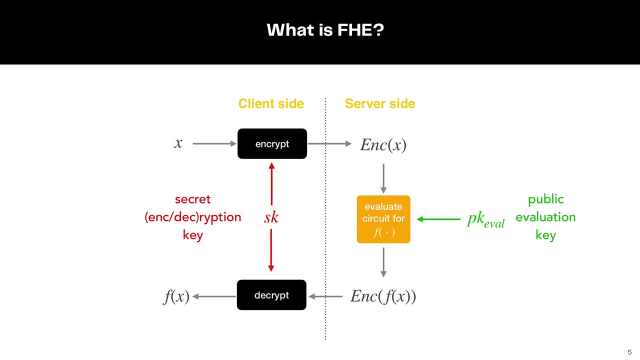 The data is always protected during transport, For example, if you think about HTTPS and stuff like that- But the data is encrypted. The data is actually in the clear on the server side. What FHE allows us to do is to keep the data encrypted during the whole process. 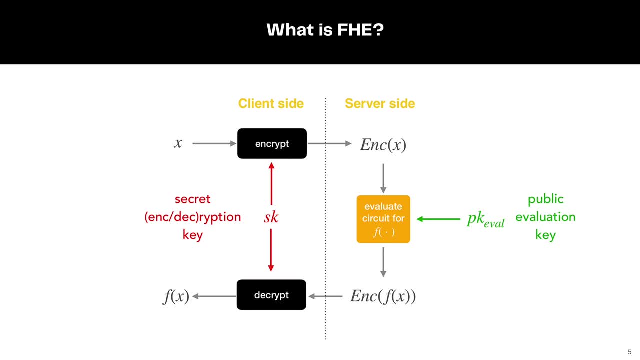 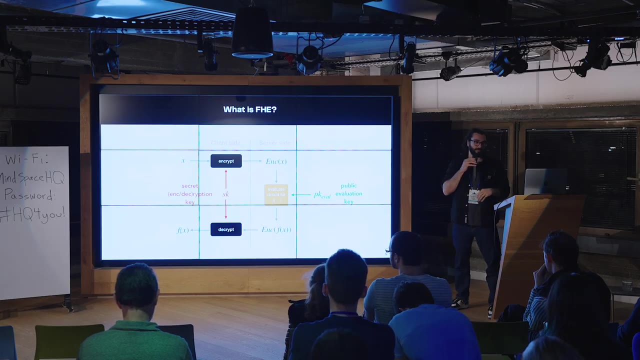 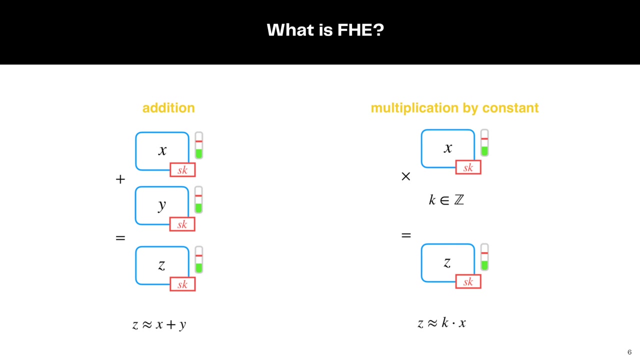 So even the computation is done on the encrypted data. That allows a lot of use cases like the ones that I talked about, where actually the model, which is actually just the function F that we are applying here to the encrypted data. So at XAMA we are using TFHE, which allows us to do three basic operations. 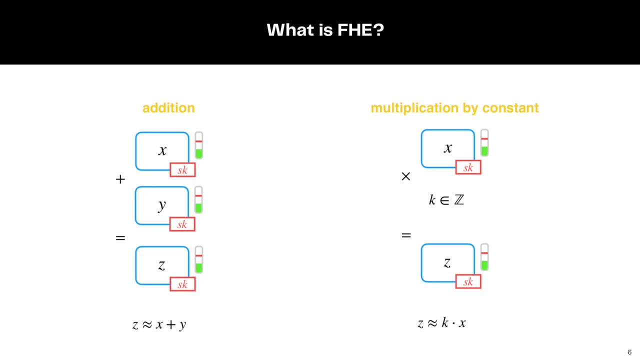 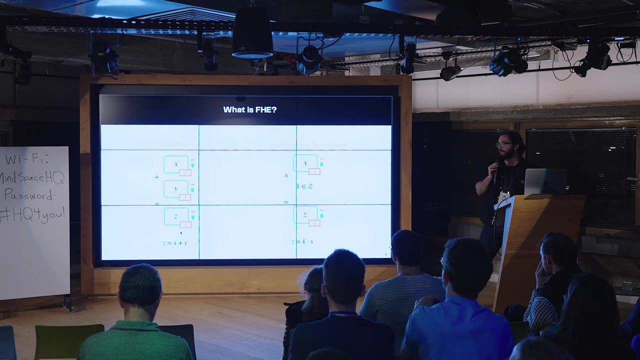 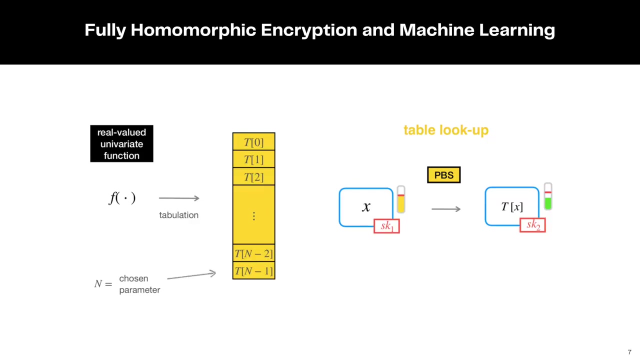 But those operations are actually all we need to do: privacy-preserving machine learning. So the first operation that we can do is additions between ciphertexts, And then we also have multiplication by constant, And the third one is actually the most interesting one, because it's 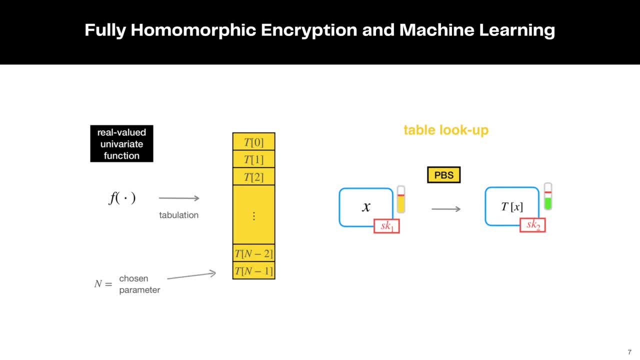 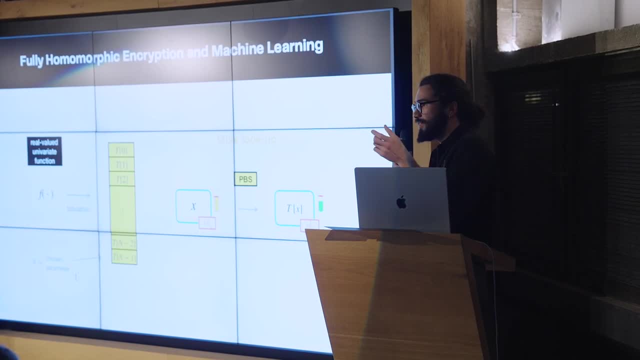 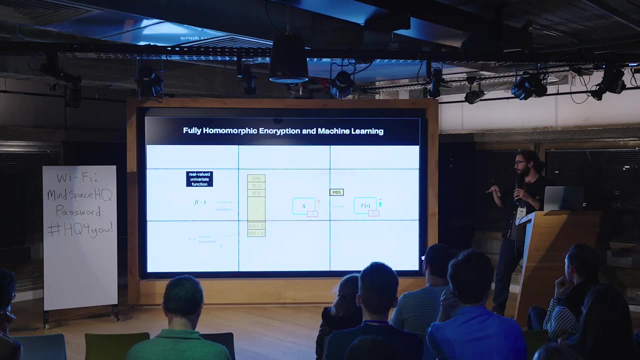 it's basically a PBS or table lookup, according to which community you are talking to, And it basically allows you to do a table lookup on data. So this is kind of the same thing as evaluating an univariate function on the data. There are also nice properties for like noise stuff. 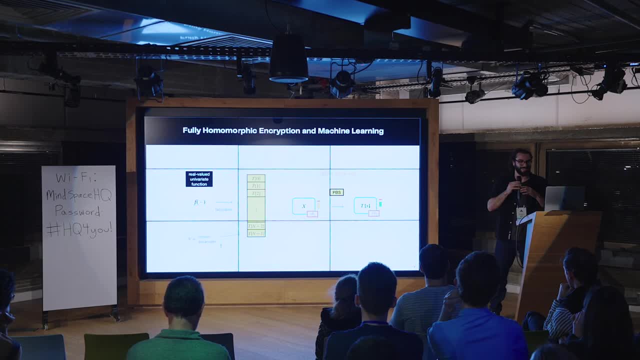 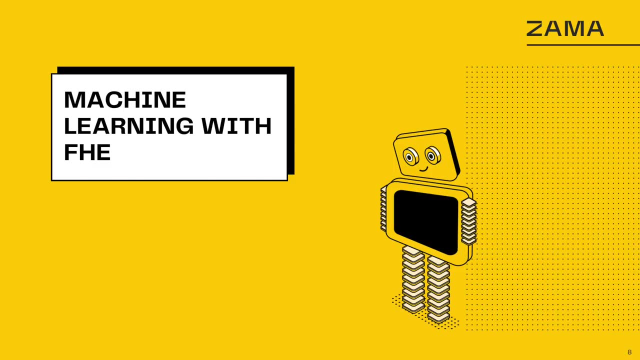 I won't go into that since, as I said, I'm not a crypto guy, So yeah, So how can we use those properties to do machine learning? And this is like the main thing. This is the main topic of the talk. 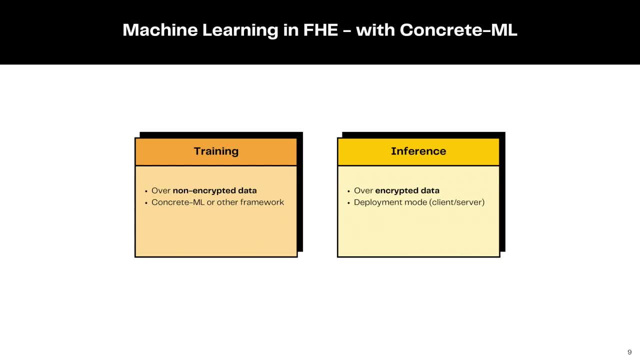 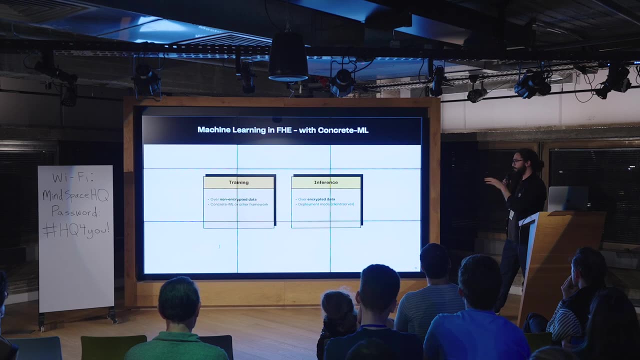 So, with what we do at XAMA, we are focusing on the inference side of things. All the training is done on clear data, Or you could use another method to do privacy-preserving training, like federated learning or other methods. What really is our focus at the moment is to do the inference and to provide basic APIs. 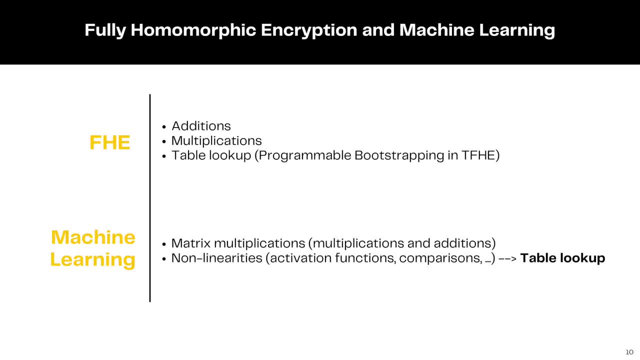 so that data scientists can do this kind of stuff. So yeah, As I said, we had basically three types of operations in FT, So we have additions, multiplication and table lookups, But actually in machine learning we are mainly doing two operations. 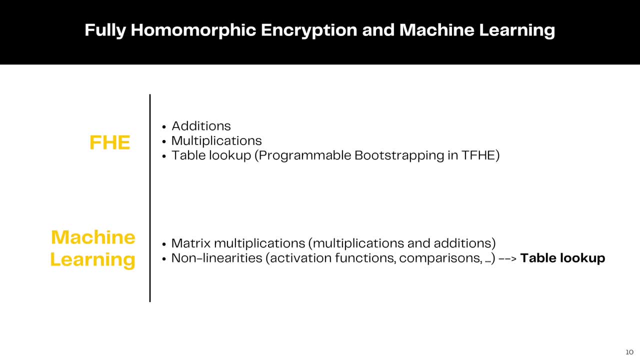 which are matrix multiplications, which can be done with the additions and multiplications, And then we have table lookups that are actually quite useful to do nonlinearities. So if you are thinking about deep learning models, they are basically just a combination of those operations. 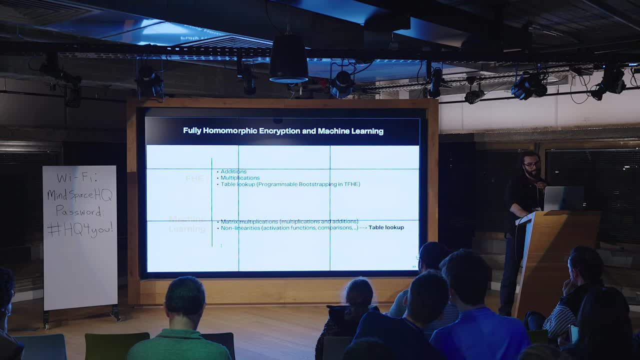 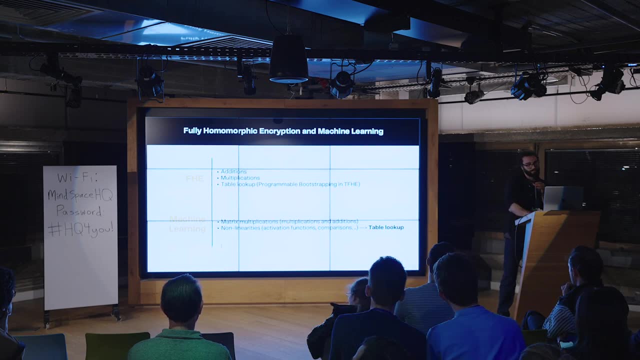 So nonlinearities and matrix multiplications. Okay, Thank you, Bye Bye, Bye multiplication. So we have all the tools that we need to actually do machine learning: model inference in FHE. The only thing is that we have to convert our model. it could be like: 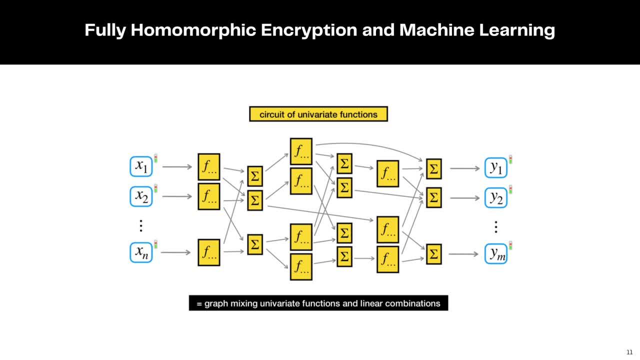 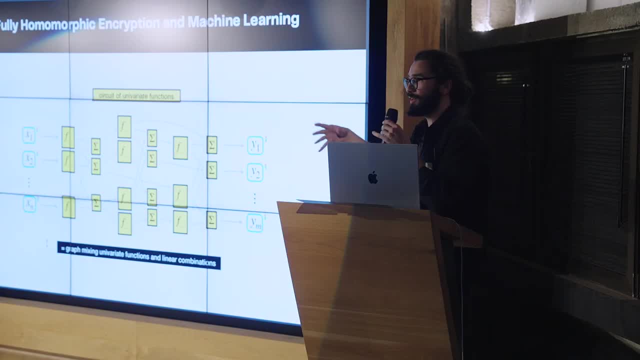 a tree-based model. it could be a neural network, anything to a circuit, and if you think about it like this, kind of circuits are very similar to the things that we manipulate when we do deep learning. This is basically a chain of operations like matrix multiplications and. 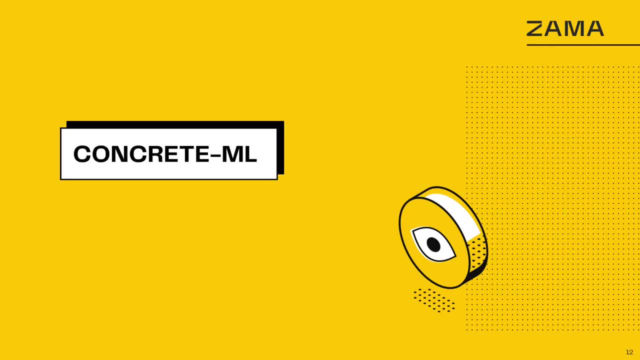 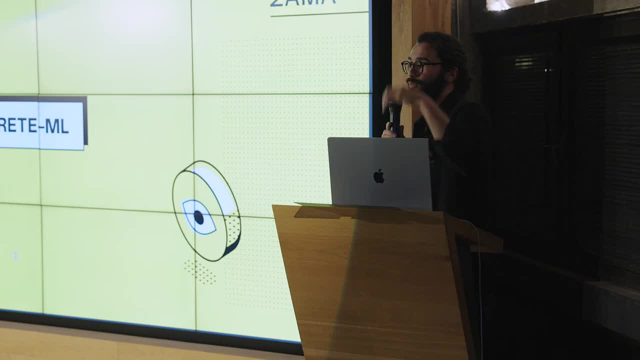 as I said, activation functions. So, more concretely, at XAMA we have a whole stack called concrete and we sit on top of the stack and we provide a library that's called ConcreteML. that basically provides all the APIs that someone needs to do machine learning in FHE, The main objective, 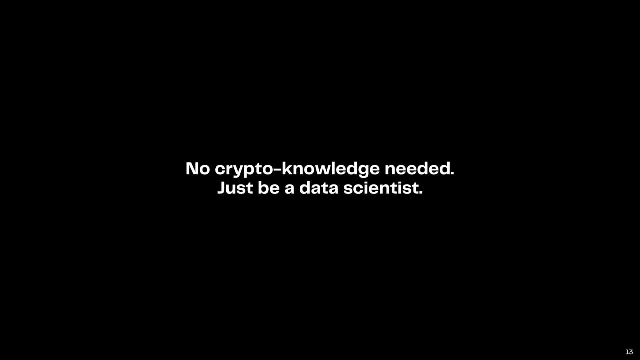 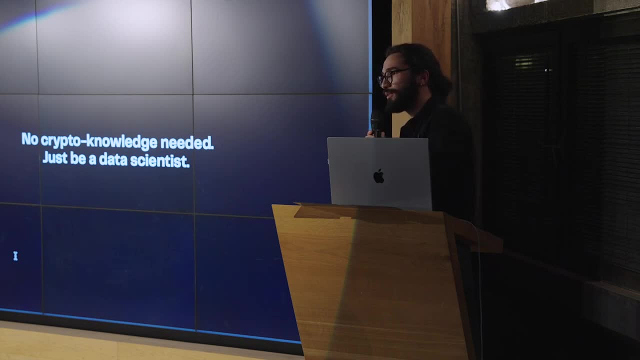 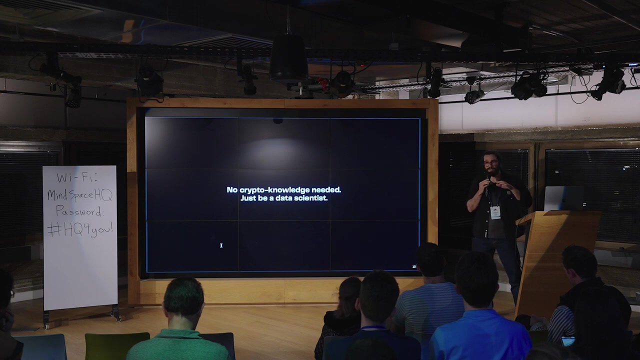 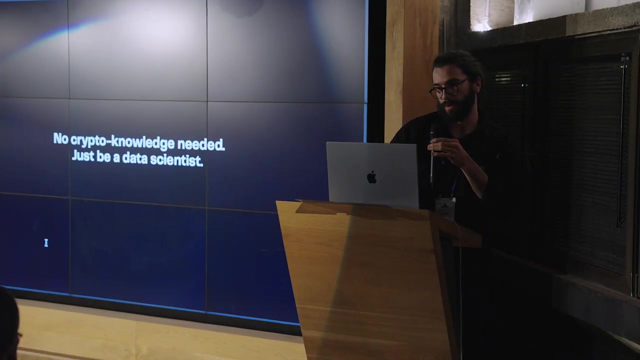 of the library- which is open source, by the way- is to provide all the APIs so that a data scientist can do FHE- inference of machine learning models- without any prior knowledge in cryptography. So, basically, even myself I have a basic understanding of how TFHE works, but still I'm able to develop the library and actually use it To do this. 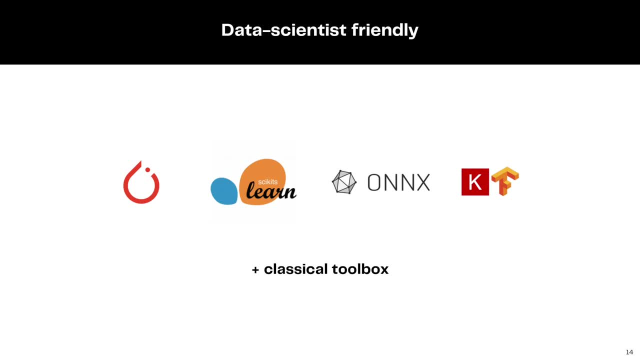 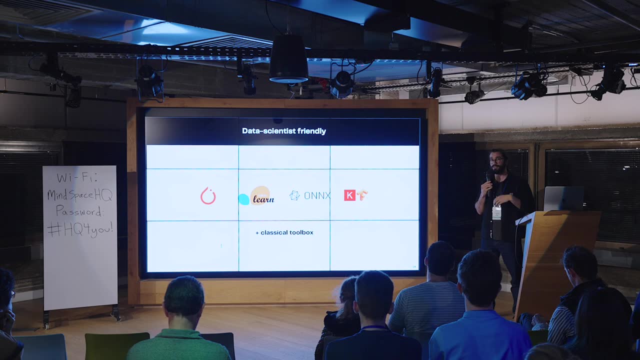 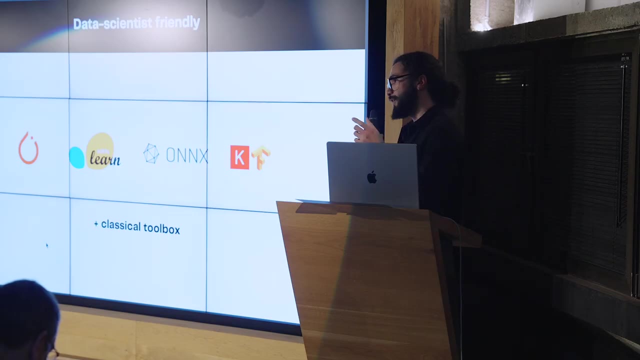 we took inspiration in well-known machine learning libraries, So Scikit-Learn is one of the most basic libraries that you can find to do machine learning. It exposes simple APIs so that anyone can do it right, And then we also support more like complex frameworks that do deep. 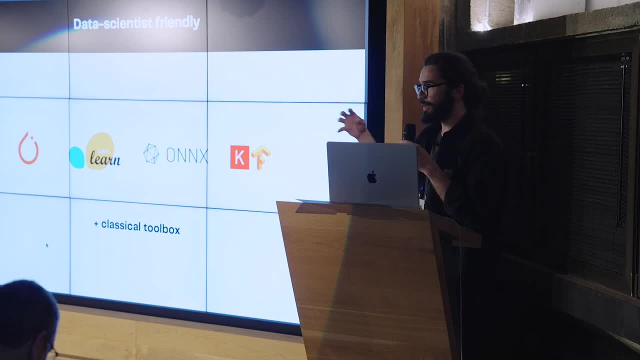 learning like by PyTorch or TensorFlow, And we provide APIs that plugs onto like these kind of libraries so it is super easy for data scientists. It doesn't have to re-learn everything to do machine learning in FHE. One of the drawbacks of FHE as we use it is: that it has a lot of features. For example, it's not a big deal because we have a lot of data in FHE and we have a lot of stuff that we can use in FHE and we don't have to do all the small things that we have to do in FHE, in FHE. So we have a lot of little things here. 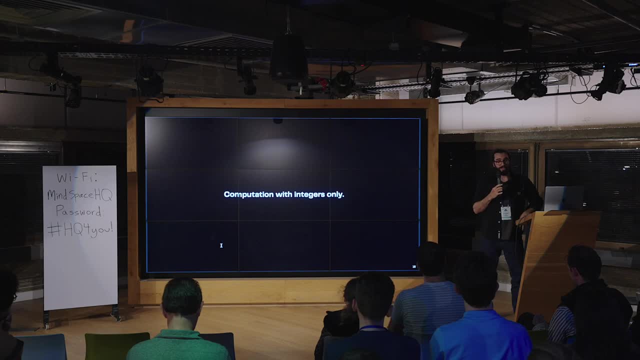 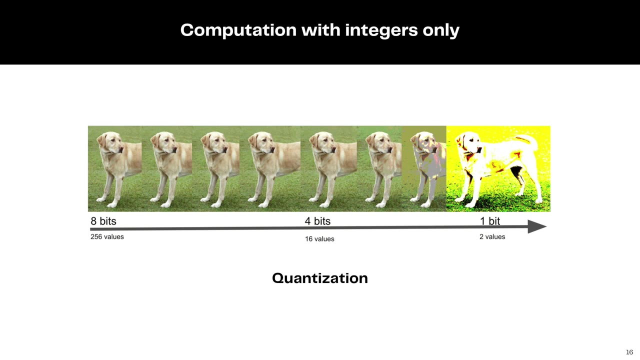 is that we can only do computations on integers. but that's actually not an issue, because there is a whole field in machine learning called quantization And this was at first developed for embedded systems where you actually have a lot of constraints on the memory, on the. 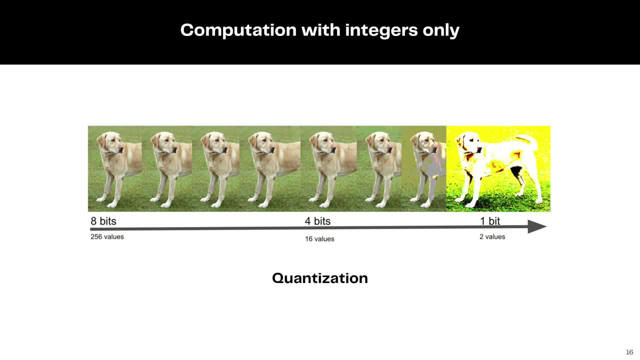 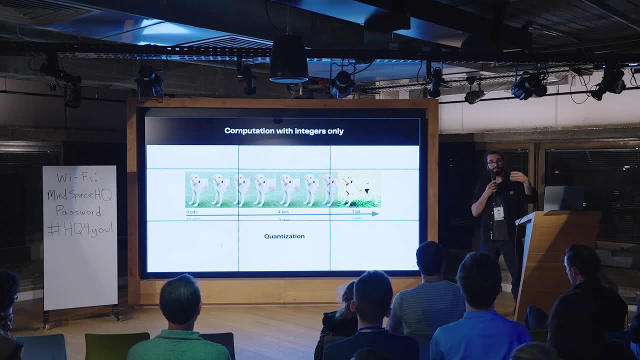 system where you are running your model. But all of this literature is actually quite useful for us because since we do everything on integers, then we can take inspiration from what was already done and just apply it to FHE. So for those that don't know what quantization 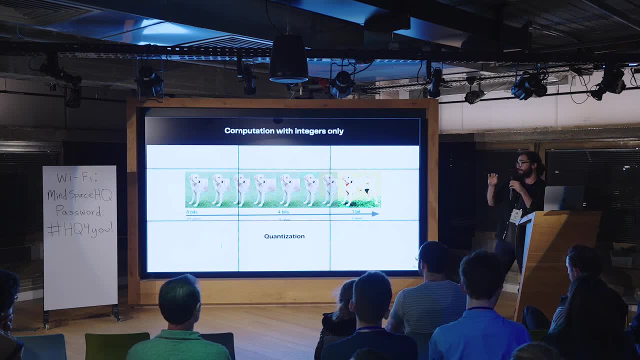 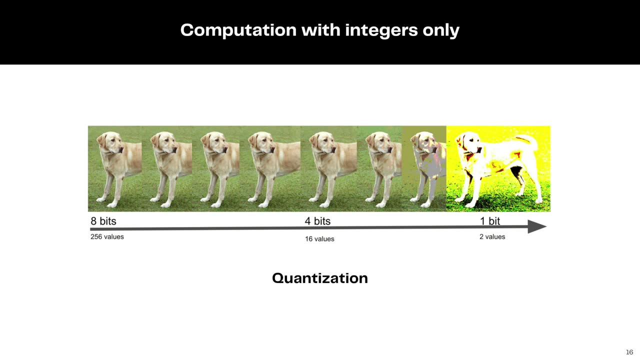 is, it's basically just reducing the bit width of the data. So here you have an example of how it looks like on an image of a dog, And actually a lot of machine learning applications right now are based on images And, as you can see, even with one bit quantization- which 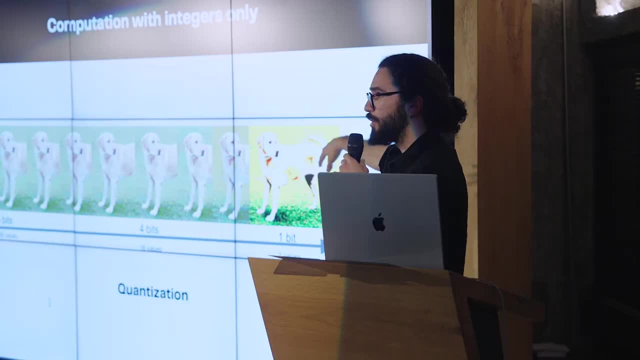 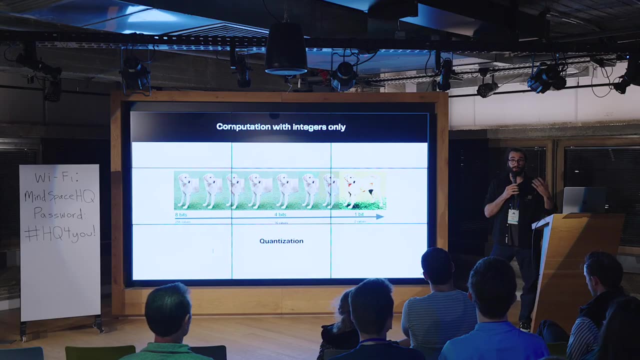 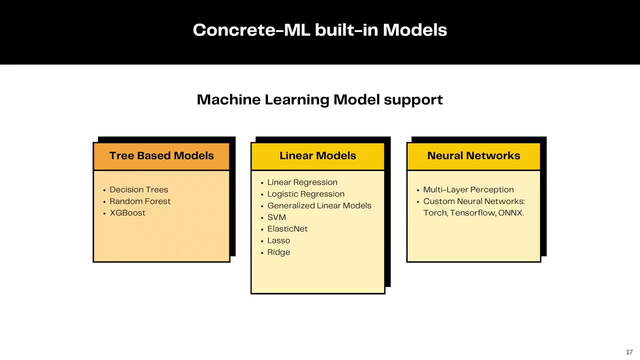 is like the most aggressive thing that you can do. you can actually always see the dog right. So the idea is that if we as humans can still see the dog, deep learning models should be able to also perform nicely on this kind of data, And actually it does. So we provide. 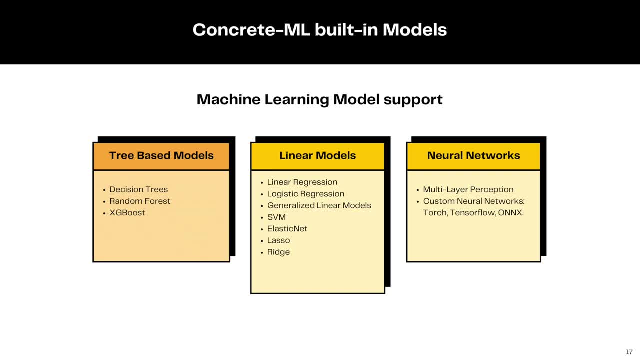 different levels in ConcreteML. So a lot of support for typical models, like more classic machine learning models, like tree-based models, so decision trees, random forests and exoboosts, And then also a lot for linear models And then also a lot for linear models. 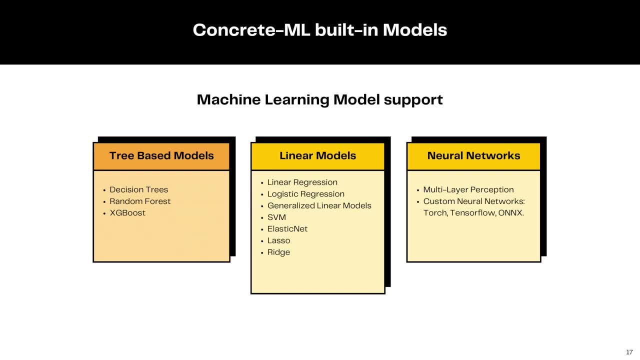 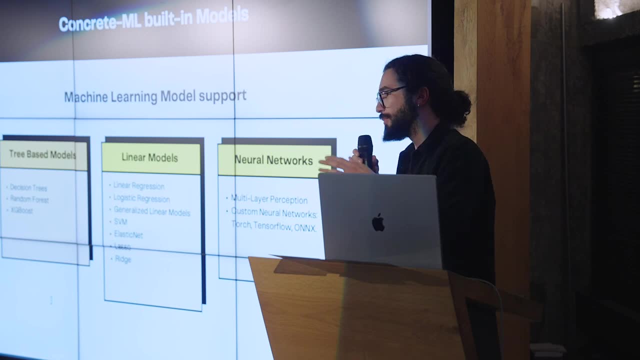 And then also obviously neural networks. So we have simple APIs where you can have like a simple MLP already done. And then we also provide stuff for data scientists that do a bit more advanced machine learning. so that can come with I don't know super complicated deep learning model and then convert it to 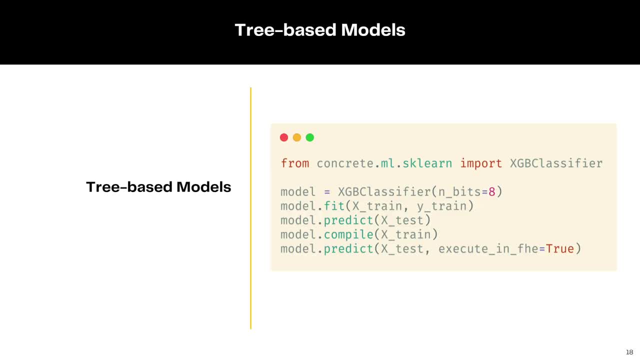 FHE, As I said, the main idea is to be really as simple as possible as possible. So if a model is going to be very, very complex, we've got to make sure that. if it's going to be a very complex model, we've got to make sure that it's going to be not just a simple model, but 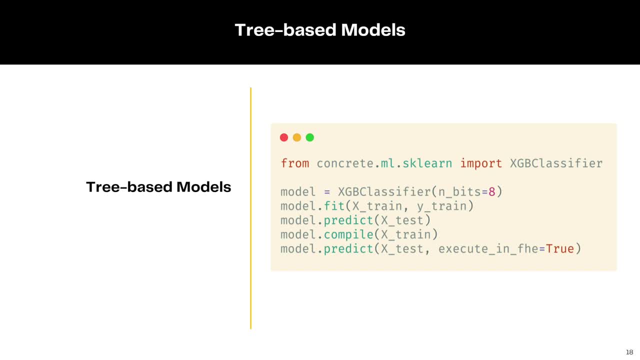 as possible. So here you can see. it takes I don't know six lines of code to train a model and run it in FHE. So the only difference with the basic APIs of machine learning, if some of you are familiar with that. 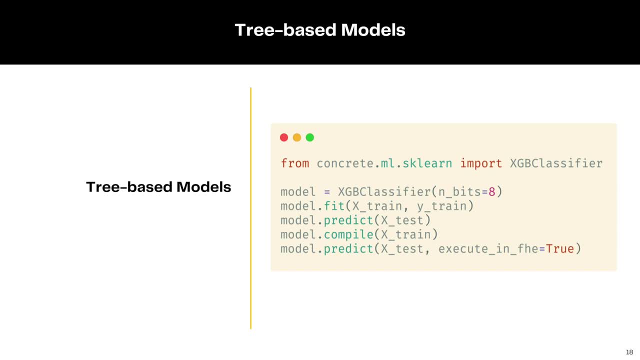 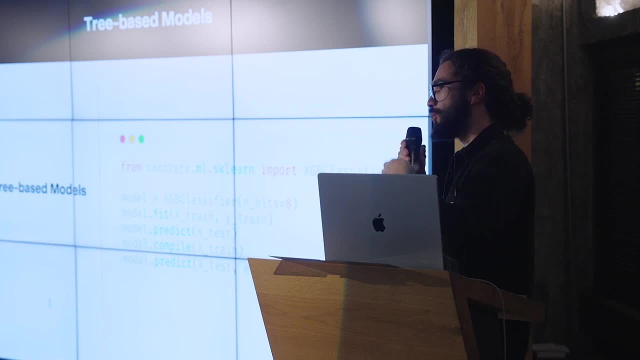 is the n-bit parameter here and the execute in FHE. So the n-bit parameter is used to do the quantization of the model. so, under the hood, the model we train on context data and everything is handled for the user, So it doesn't have to preoccupy itself. 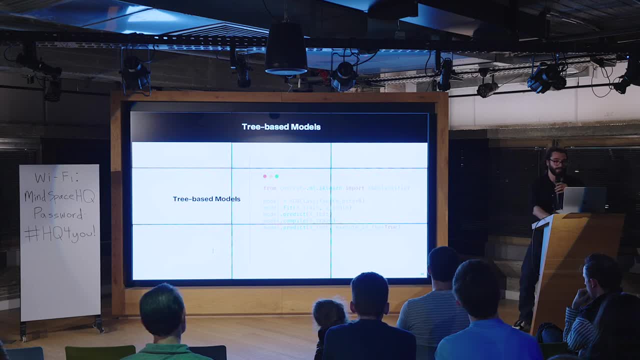 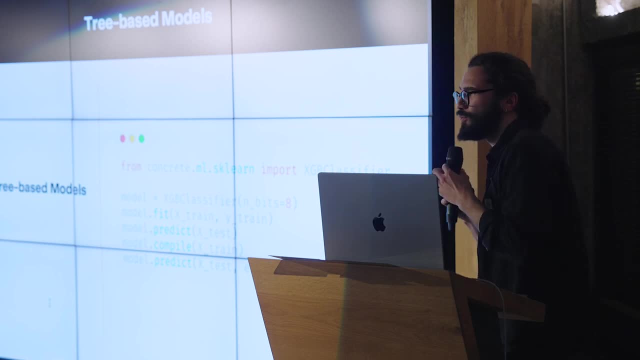 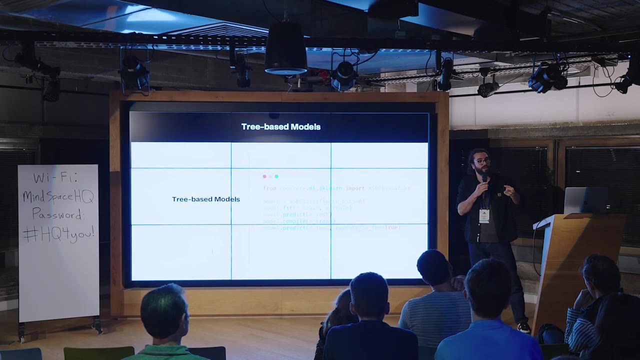 with any of those considerations? That's a good question. Actually we don't. I think it would be super complicated to do, because then you have like contamination of the model. So if you just train your model with encrypted data, then the model becomes encrypted with the key of the user. 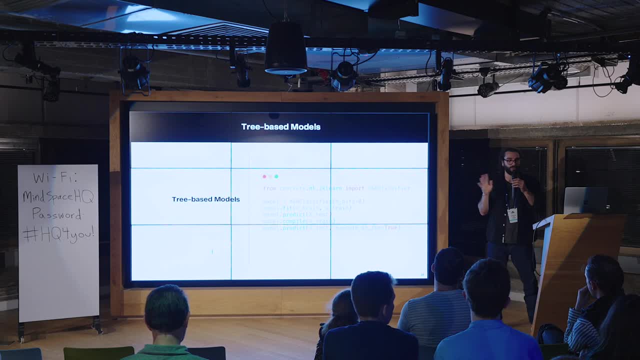 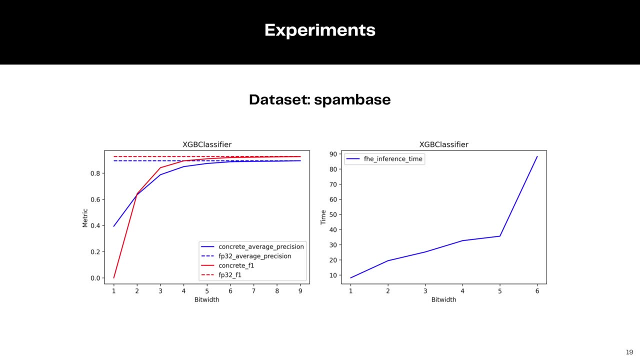 which is not a nice property, right? So there are probably other ways to do, but yeah, I don't want to know. So we provide some examples in the library, and one of them is a classification problem, And what we actually show here is that 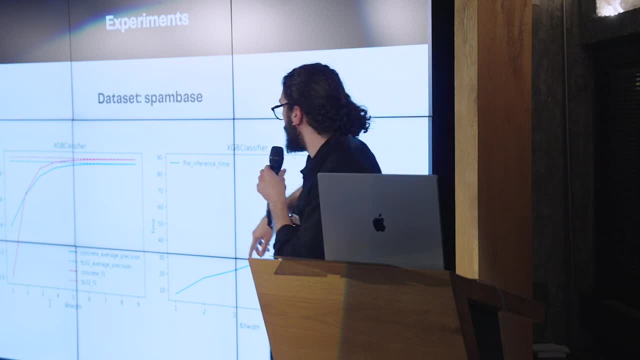 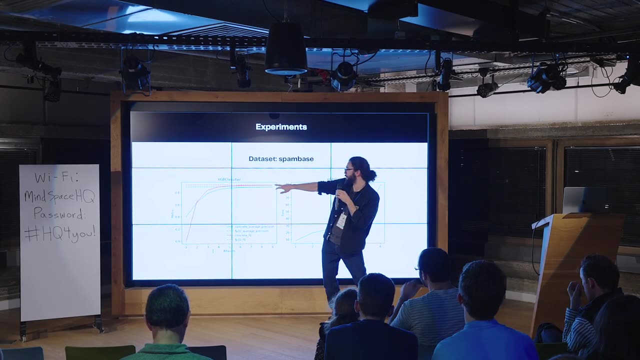 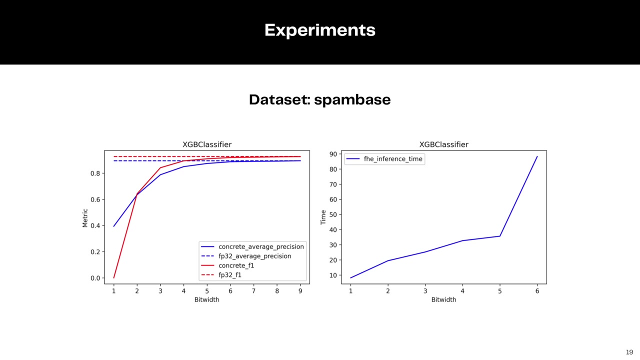 even with aggressive quantization. for example, here we have a floating point model in blue and we have no. the floating point are the dashed lines and we have the quantized equivalents in, like the other line, And what we actually show is that even for like five bits, 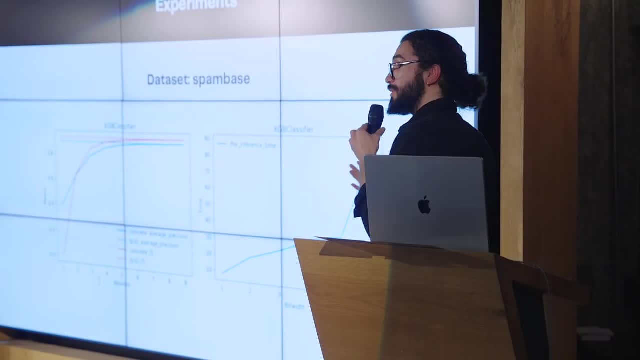 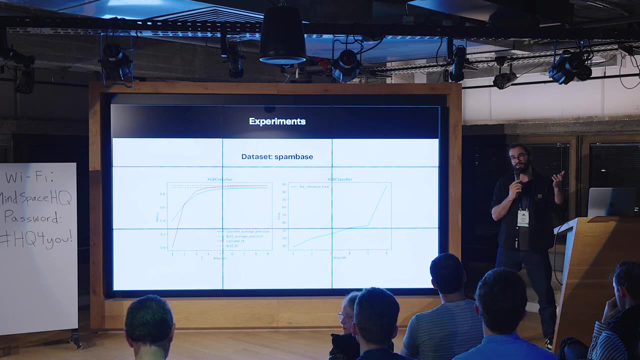 we actually reach almost the same performance as the normal model, which is a nice property. The only drawback, obviously, is that there is the inference. time is longer than a normal model, obviously, But then if you stay with low bit width. 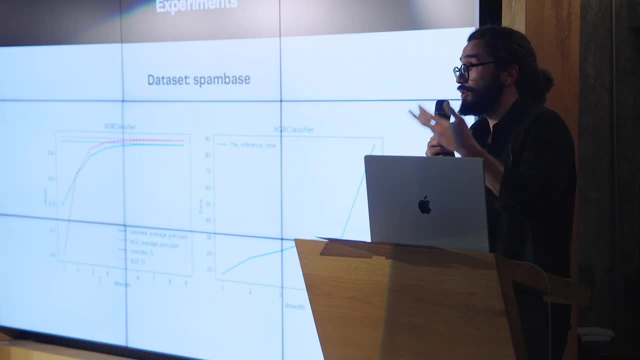 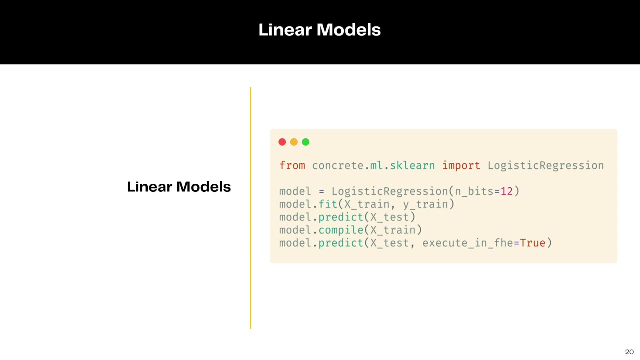 you still have decent run times and it's actually- I mean, you can actually run it on a laptop and it works super fine. Same as trees, we have also linear models. basically the same things. The APIs are the same, so it's easy to use. 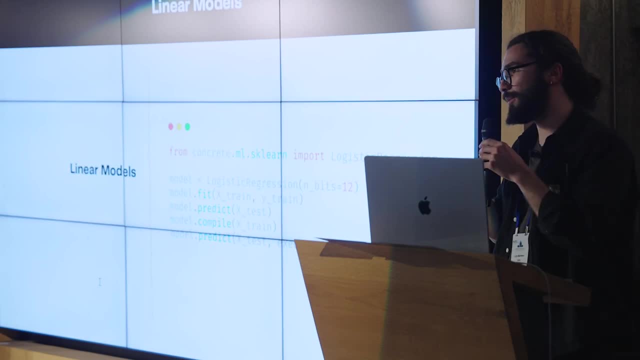 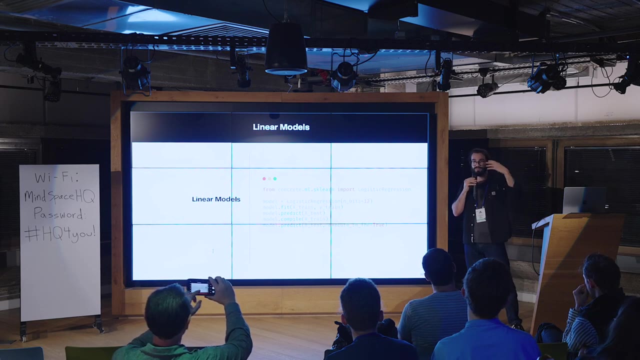 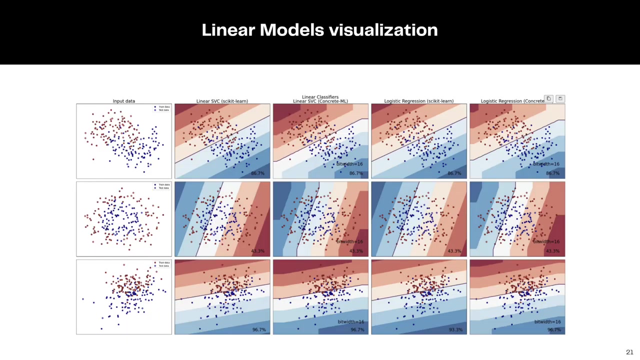 We do have more flexibility on linear models, because since we don't have nonlinearities, we don't need a table lookup and thus we can increase the bit width a bit more. So that has nice properties, because then you can do a bit more complex stuff. 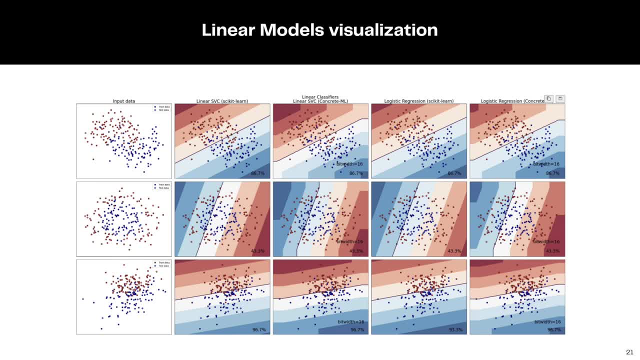 Here, as you can see, the okay. so here we are, comparing scikit-learn models that run on floating point values and concrete ML. The concrete ML ones are those and, as you can see, they are like small quantization artifacts. 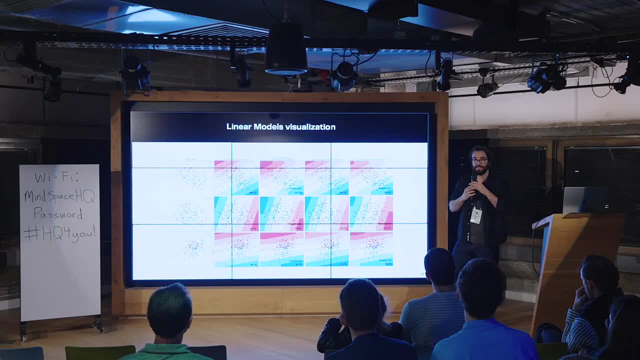 on the decision surface, but they are really small. The only place where they really happen is when they are not like on the support of the data. but actually, if you are doing machine learning for these type of models, you are usually trying to, you know. 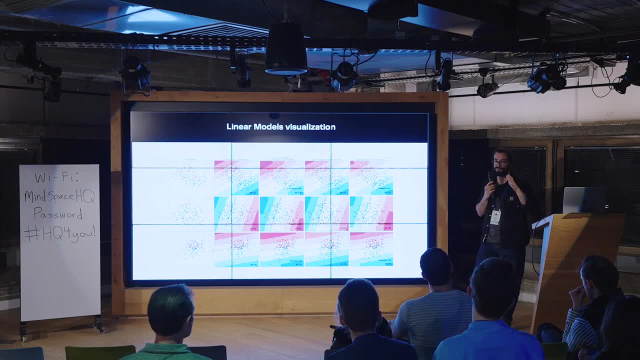 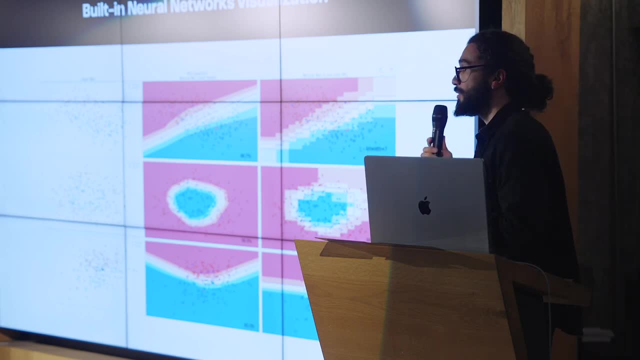 for these type of models, you are usually trying to, you know, for these type of models, you are usually trying to, you know, to interpolate and not extrapolate, so that's not so much of an issue. We also have non-networks, so these are built-ins. 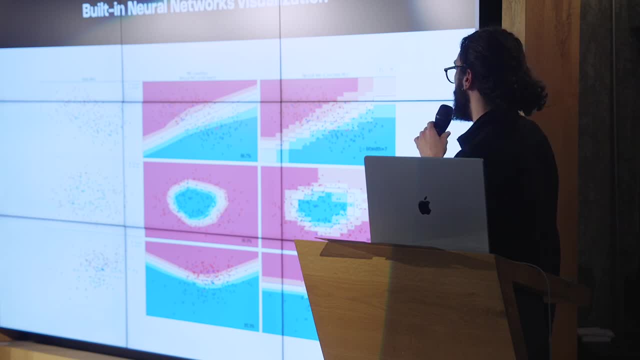 You can do them also in like four lines of code. And here we can see that we have strong quantization artifacts because we are using a lower bit width, right. But the thing that is interesting is that even with those quantization artifacts, 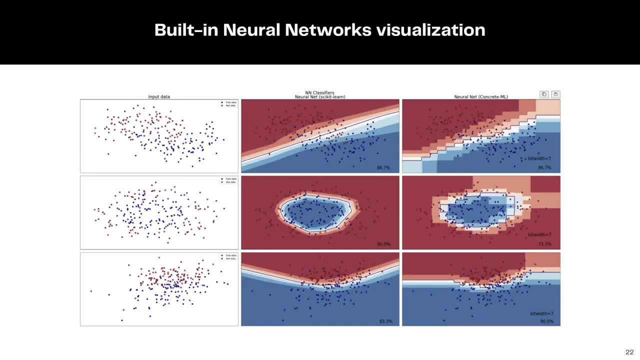 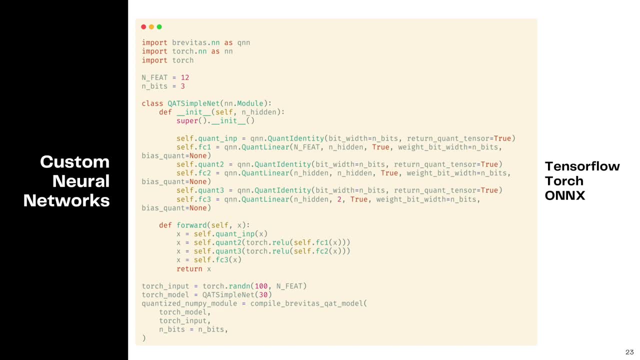 we still don't degrade the performance, the overall performance of the model. So if you take a look at the accuracy, you have very similar results. And then, last and foremost, we have support for custom non-networks, so you can come with a model. 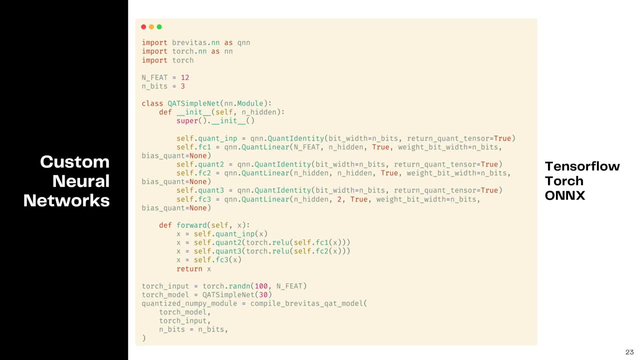 and then just plug it to a concrete ML and it should work. There are obviously like two different things when we are talking about non-networks and quantization. You can do what we call post-training quantization, where you actually take a model that's already trained. 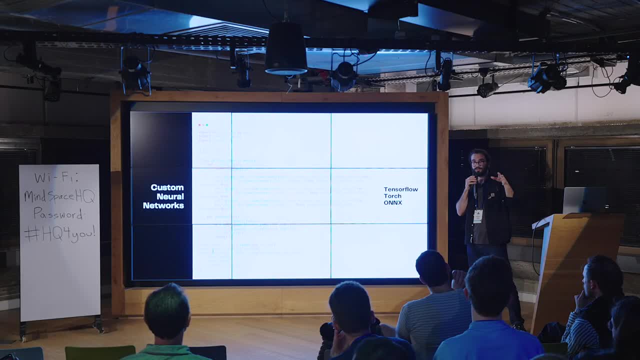 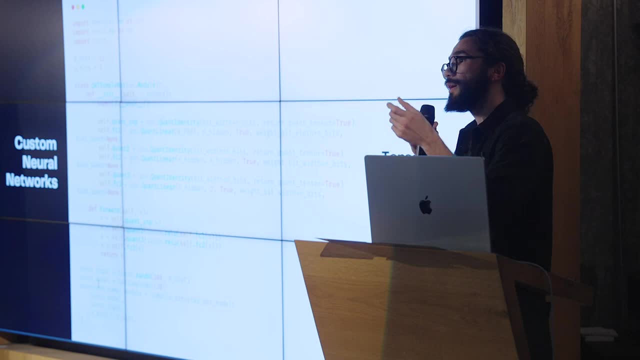 and try to convert it to low bit width. That's something that works, but there is a more efficient way to do it, And the more efficient way to do it is to either fine tune or return the model, taking into account those constraints. 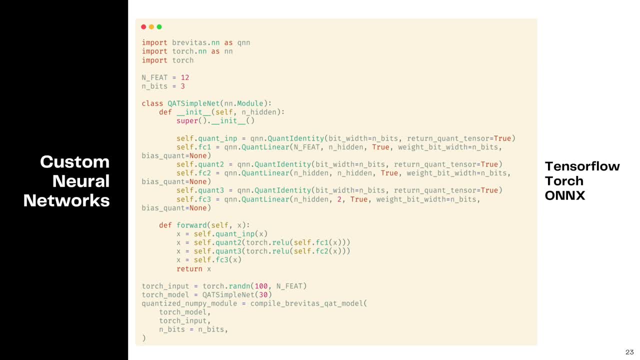 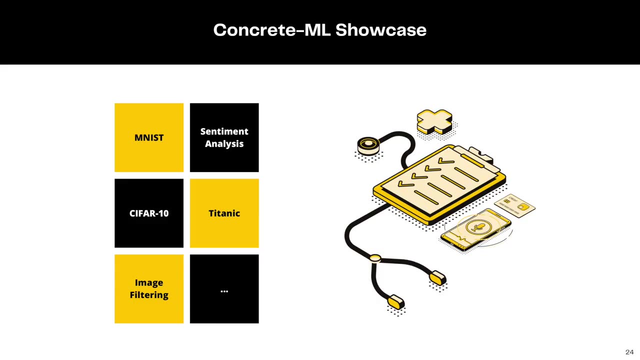 and then you have much better results. But if you satisfy those constraints, then you can just come with your Torch model, plug it into concrete ML and it will work. We have a lot of examples in the library, so we do NIST and C410 showcases. 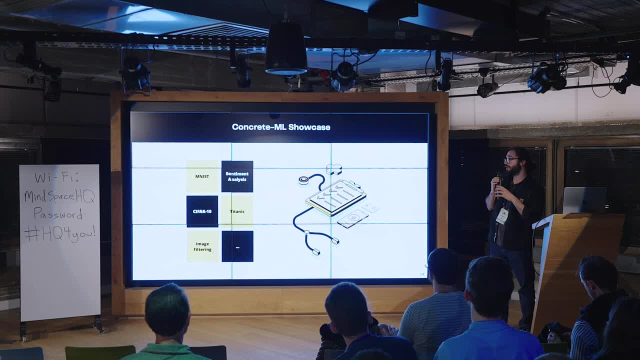 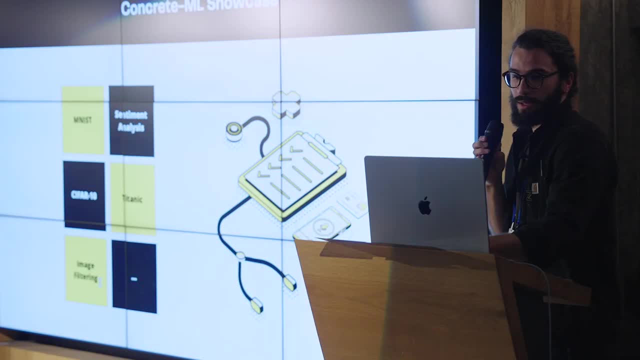 which are image classifications. for those of you that don't know, We also have an example on how to do sentiment analysis and image filtering on encrypted data, And we are trying to provide more and more examples so that it's easier and easier for data scientists. 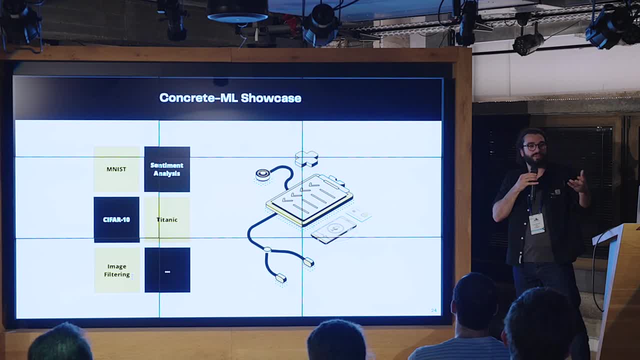 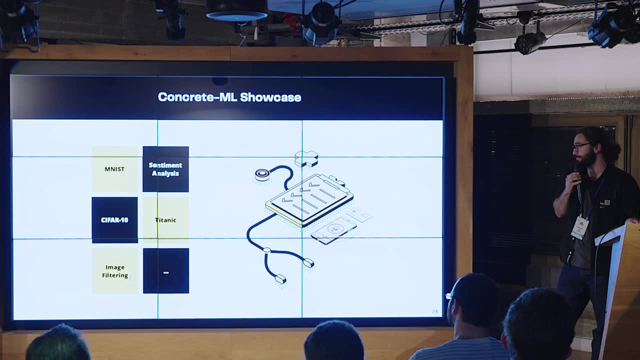 to just come like take a look, see, okay, so this is super similar to what I know, and then just like copy-paste, maybe, or like adapt everything to their need. So, in summary, we use FHE to guarantee privacy. 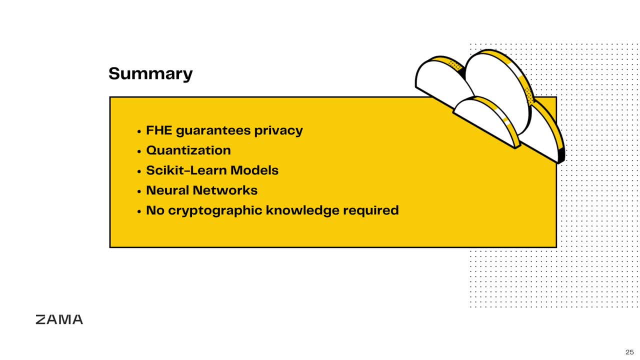 at inference time. So this is like the core of the technology. It comes with the constraints that you can only do integral computations, but luckily for us there is a whole field that already exists on topic so we can do like scikit-learn and neural networks. 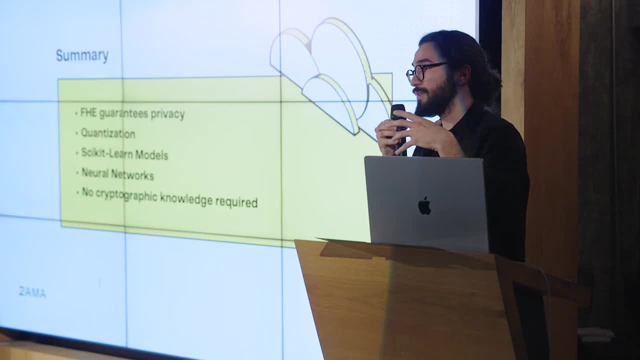 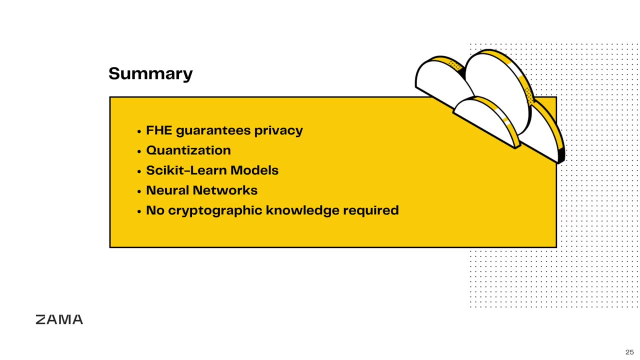 super easily and we package this so that data scientists don't have to worry about those considerations and they just can use it. And actually I think you guys, even if you didn't do machine learning before, you, could be able to use the library. 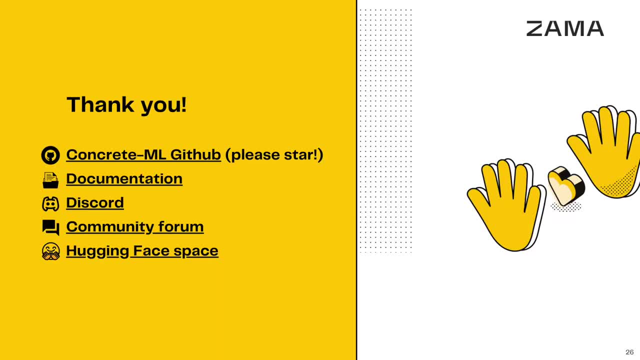 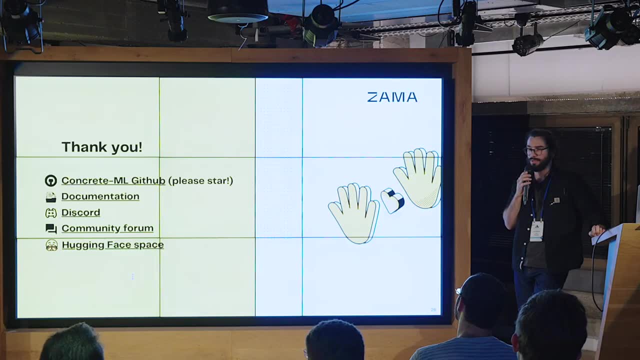 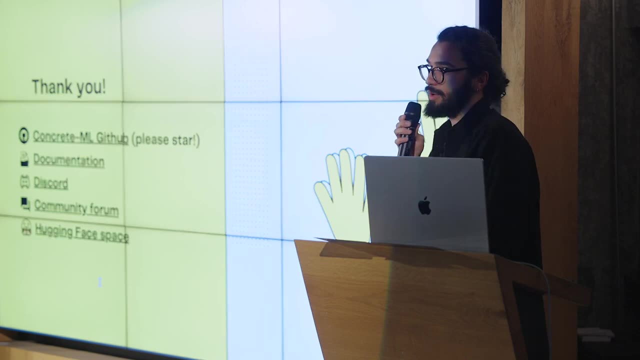 Should be pretty easy. Thanks for your attention. You can find us on GitHub. We have almost everything open source. We have heavy documentation as well on all those problems. We are super active on the FHEorg Discord, So if you have any questions, you can also find us there. 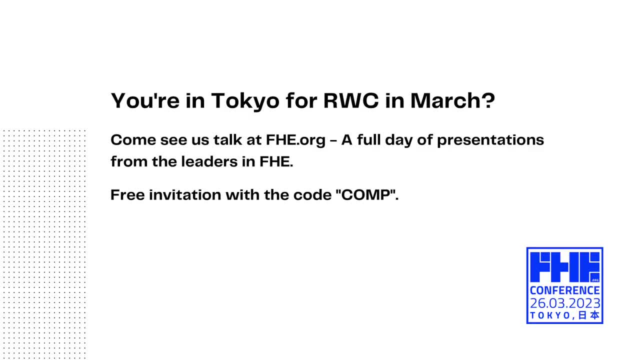 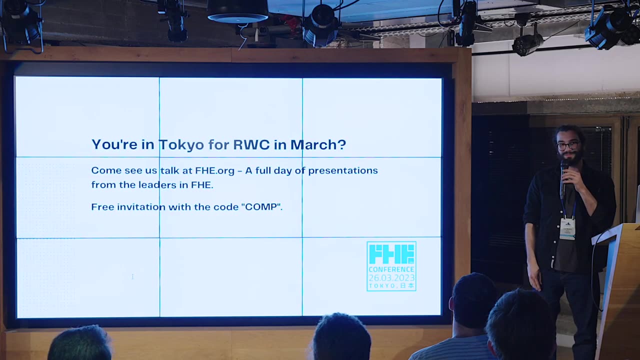 And we have a Hugging Face space. And one last thing, sorry, If you are going to RW3 in Tokyo, we will be there as well and we will be representing Concrete ML and other libraries, And you have a free invitation with this invitation code.